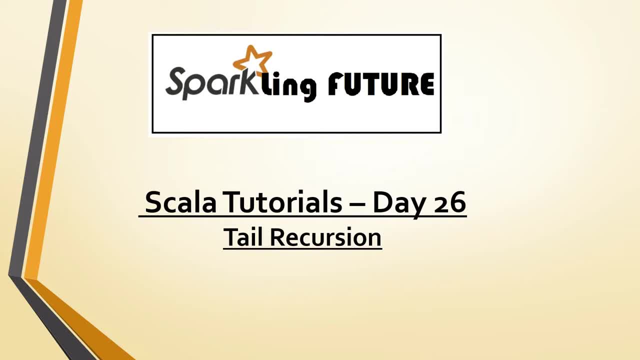 So usually recursion means. recursion is a method which breaks the bigger problem into smaller sub problems and it calls itself for each of the problem. Actually, it simply means that function calling itself that is called as recursion. So in Scala there is a concept of tail recursion. We will discuss further about this. Okay, so we all know how traditional recursion works, right Like 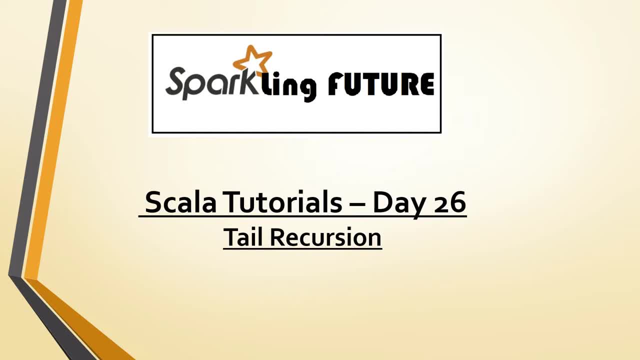 technically both are same, the recursion or tail recursion under the hood. But what exactly? computer compiles the code and the memory is managed. only that is the difference between these two, the traditional recursion and the tail recursion. And in the traditional recursion method, right, So after getting the input, like everything will have like a iteration. right? So let's say, from zero to five there is a iteration is happening. So first, after processing the first one, 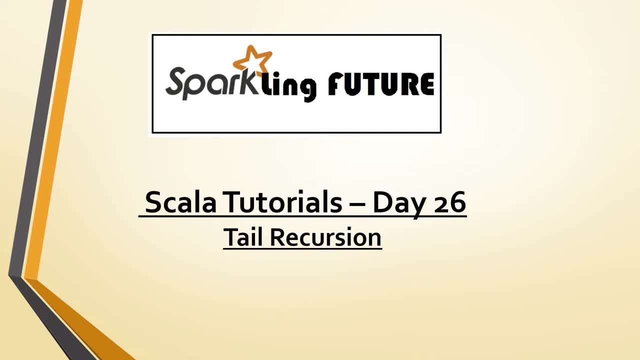 the input right, whatever is there, and it will pass to the itself. zero is there, then zero will be passed on input to this function. And again, whatever with zero or one, it would have computed some details right So that details will be saved in a stack, So that partial result. then what will happen? for example, for zero it is processing something, then it will keep it in the somewhere stack, And again it will process for the one. And till then, 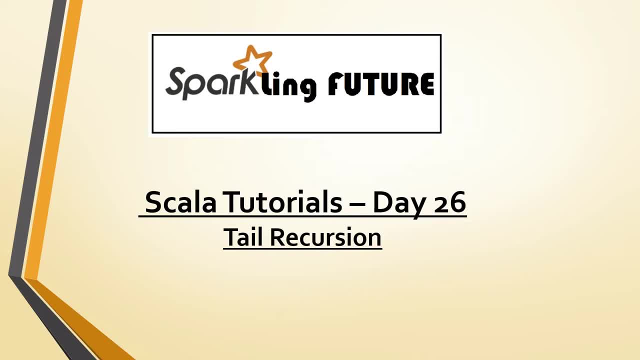 this partial result will be kept in the stack. okay, similarly, until all the entire iteration is, I mean entire loop- is completed. till then, this partial result will be kept in the stack and the finally, after the last call, the final result will be generated and sent back to the user. this is this is why, when we 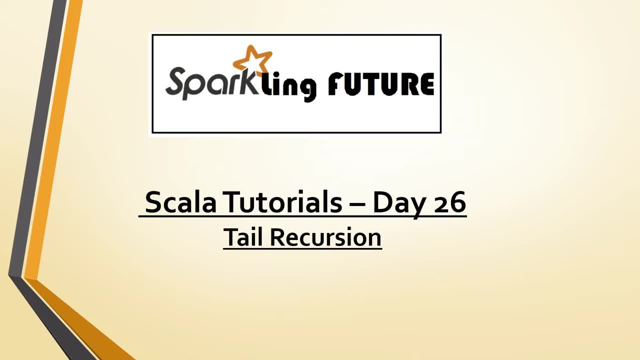 use the recursion function most of the cases. many, many of us encountered stack overflow exception. that is because of the stack uses for memory in working with the recursion. so but in tail recursion, what? what is the benefit of using it? is the partial result right, whatever is generated in the iteration. 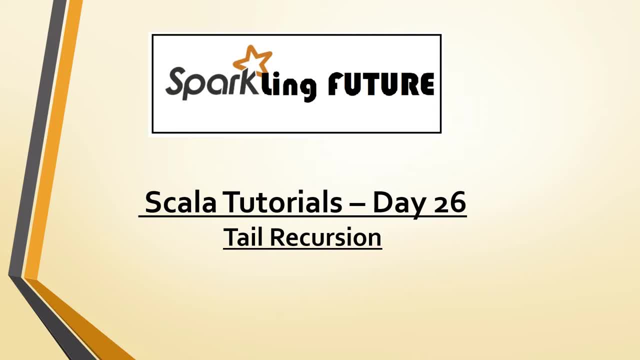 the partial result will be sent to the next call along with the input data or we can say unprocessed data. so this process follow until all the calls are completed. the final result will be sent back, which means the class don't need the stack here. okay, it's, it's. 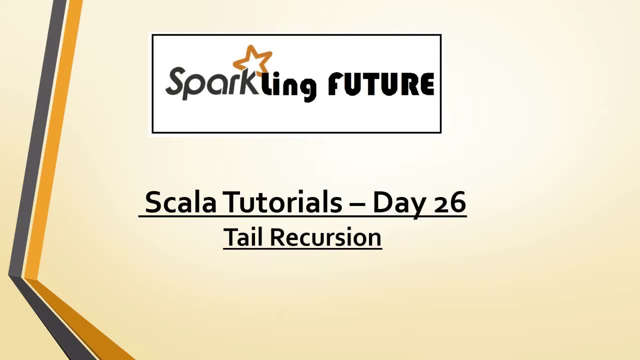 memory very memory effective. so the input itself, i mean the what is the processed partial result, will be sent as input. so because of that, it is it. it won't use the stack. that's why it is very memory effective and it it also eliminates the stack overflow exception. okay, so now this is 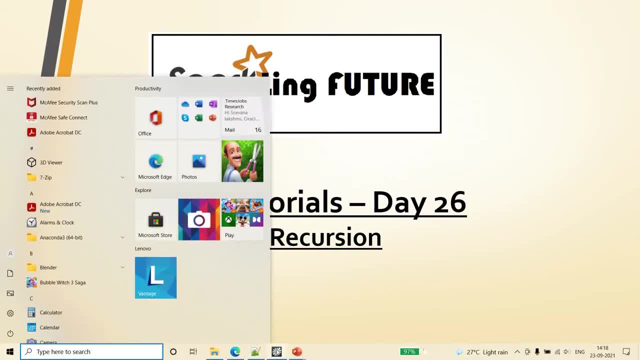 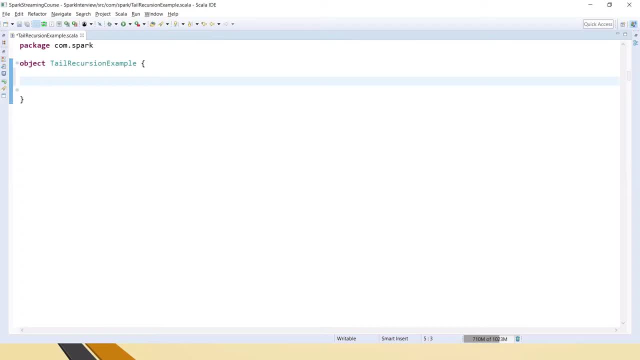 about theory, about tail recursion. now let's look into some sample code to understand this. i've just created one very simple object, okay, so now usually, for example for this right, most of most of us use fibonacci series. okay, so we will just see what is fibonacci series. 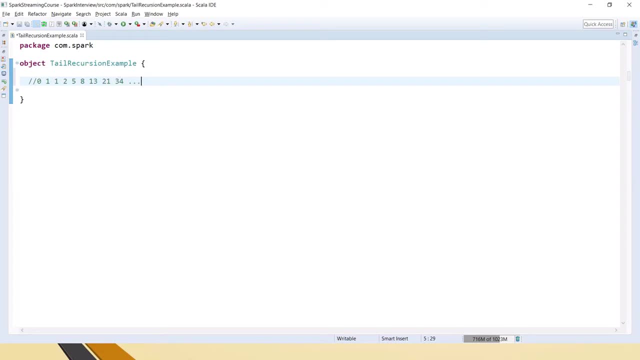 and we'll see how to solve that. so this is called the fibonacci series, which means that the previous series number and the current number, if you sum it up, it will generate the next number. okay, so for getting this one, we should sum up 1 and 1 plus 1 equal to 2. okay, so 2 plus 1 equal to 3, 3 plus 2. 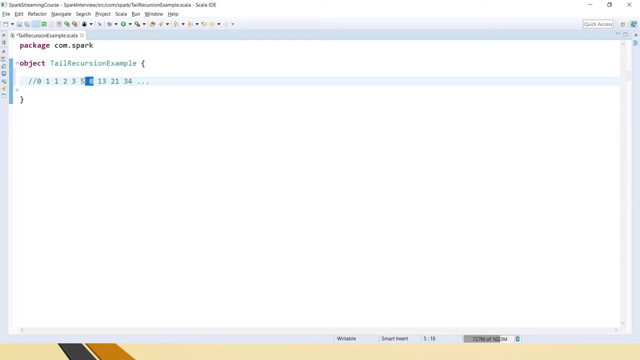 equal to 5, 5 plus 3 equal to 8, 8 plus 5 equal to 13, 13 plus 8 equal to 21, 21 plus 13 equal to 34, and so on. so this is called as fibonacci series here, if you notice a for every current number. for every current number, we have to sum the. 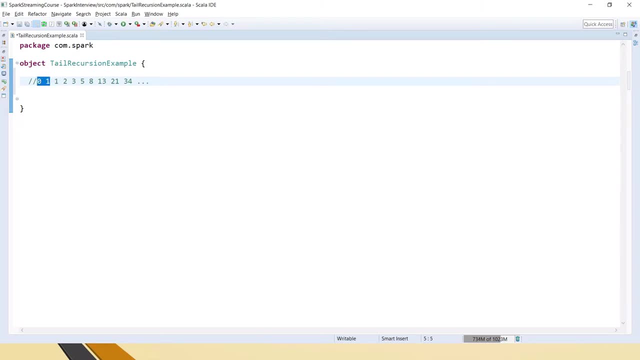 minus 1 and minus 2, so it's like a iterative right. every time it has to consider the previous two values and sum up with the current one, then only it, will it? it i mean manages the. it prints the a fibonacci series. so that's how it works. and if you notice here, every time it has to call. 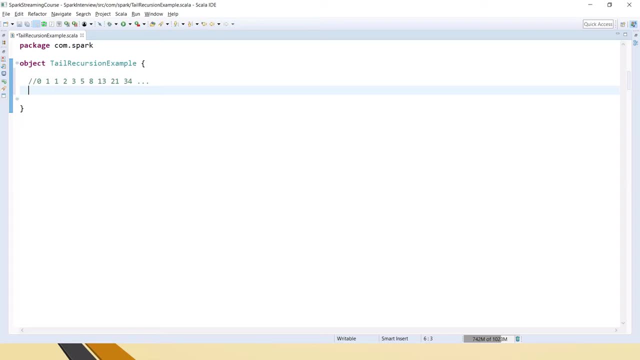 itself, right? i mean, if you write it in calling multiple functions. instead of that, we use recursion for fibonacci series usually, so now let's write the code for printing this series using the tail recursion. okay, so now let's create one method which takes the input as integer- okay, 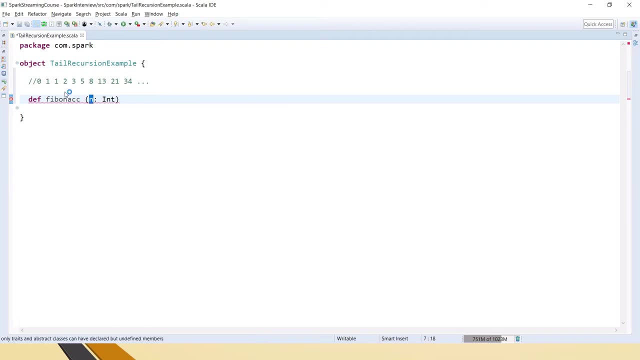 because we should say five. if i, if you say five, one, two, three, four, five, five iterations, it should complete and it should print the value. okay, so, and then returning also will be int. and now what we will do is- this is the main function for fibonacci, and because we have to use the tail, 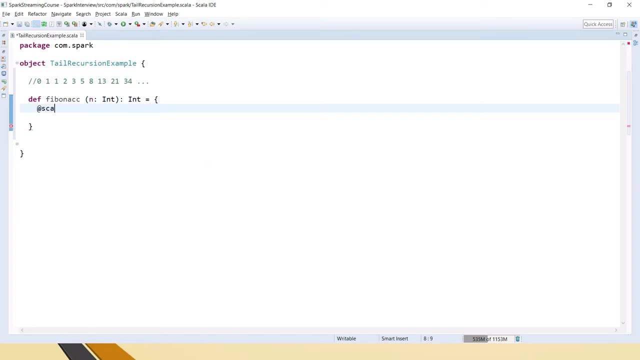 recursion functionality and we have to add this annotation. okay, what is annotation and all we will see later, but for now, you just remember this right at: at the rate and tail rec. this is the very important annotation. you have to use it for the for while using the tail recursion. now, after this, whatever we declare is the tail, 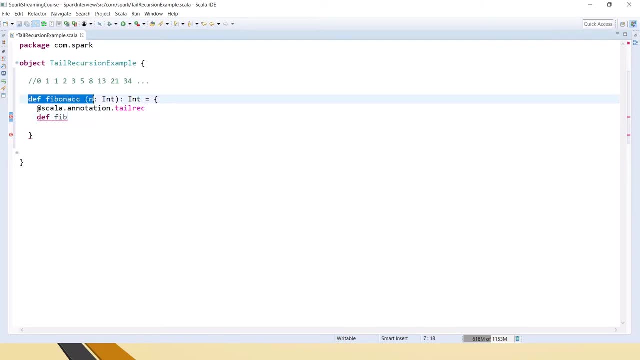 recursion function that we are using. okay. so why we have here all is, i will explain in in a minute, but let me write the code for this. so now let's have a small function called feb. okay, for this we have to pass the integer. whatever we are getting from here and we should. 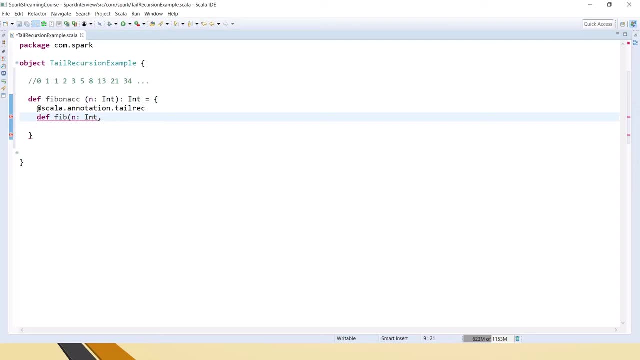 have some initial values, correct, so for that we will take it as a and b, some initial values. okay, so i will explain you that also with some example, then you can easily understand it. if you want to a simple application. so here is e zero square root of n. 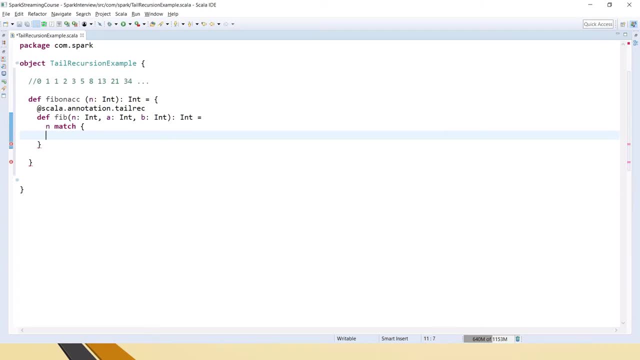 um, two zero square root of y. so you know it: long term, in common case, a or h would state that this t is equal to one, two, three and x will instead tender is equal to min a, i r, which is a slice equal one. so if you see here, if it is zero, the value of zero position is always zero. so that's why we are. 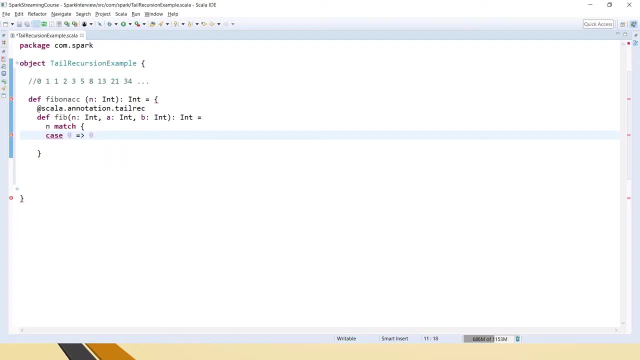 taking it as zero. okay, and then if you see that second one, also one. if you take the one, it will be one. that is because zero and one, even though we we, if, if we are sending only zero, right, then it will return zero. for example, if you are sending one in as input to this function. so what it will. 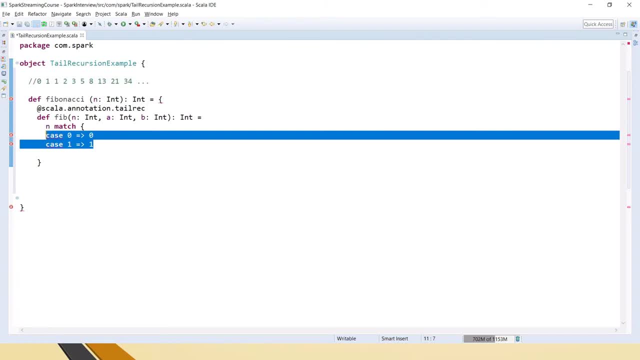 do is one and the previous one is zero. so for counting, like that we are sent as mentioning, like if the zero means take it as zero, one is take it as a one, and then if it's something else, okay, if it's something else, then what we have to do, we have to first let me print: 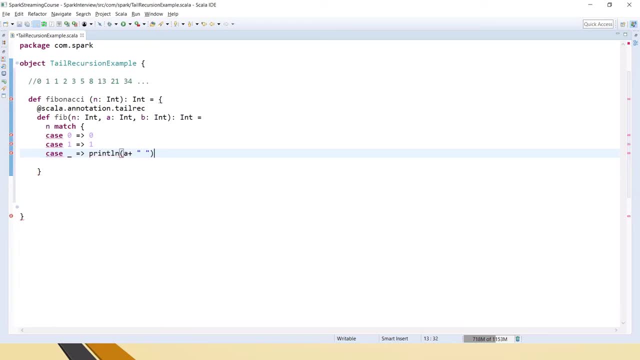 print, print, okay. and also we will call the same function again for two things. here we have to call it like: first we have to take the previous one and then b, and then we have to sum it up: the previous one and the n minus two, okay. 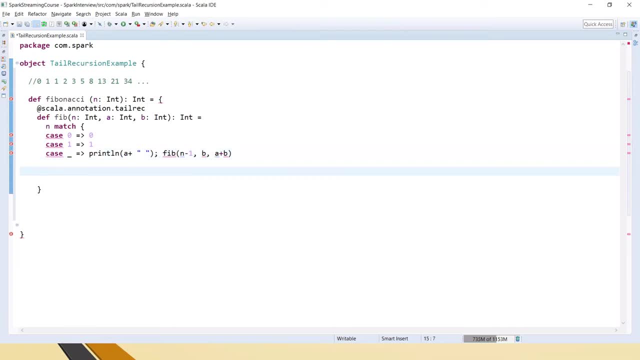 and hope this is closed. oh yeah, here it is closed. some brace is missing. okay, and n comma zero comma one. okay, for using the tail recursion. first one is using this Annotation at Tailed it and the second one is the last lin of the, the last line of the highest ranking, while the built position of the N comma 0 comma. 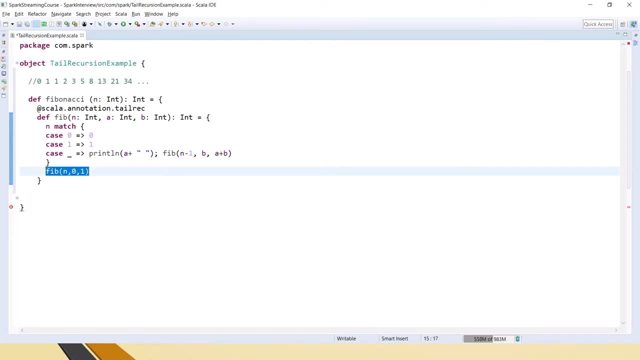 of the n comma 0 comma and n comma 1 and n comma two. also take those and the. those are the more analogous seen here. and this is not the final đây Subscribe. this paper is komenrabyorg method. tail recursion method should be the call to itself. if you notice, this is the last after. 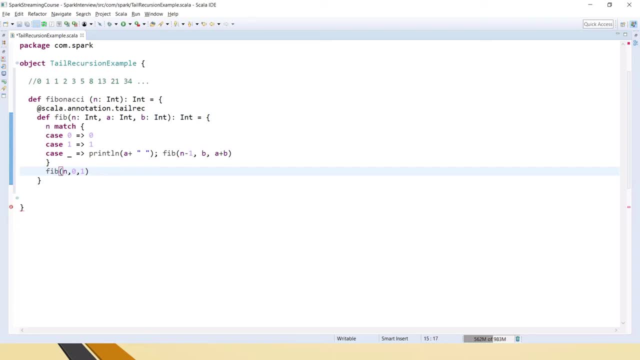 this: what if you say even the println also, it will give error saying that it it will expect this to be the last line of the method. okay, so now this is the method. so now let's write the main to run this code. let's say five, okay, so. 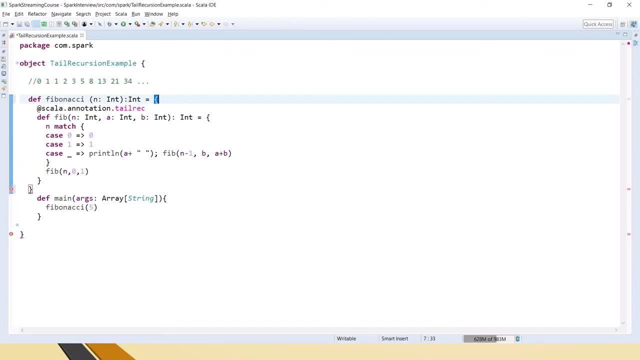 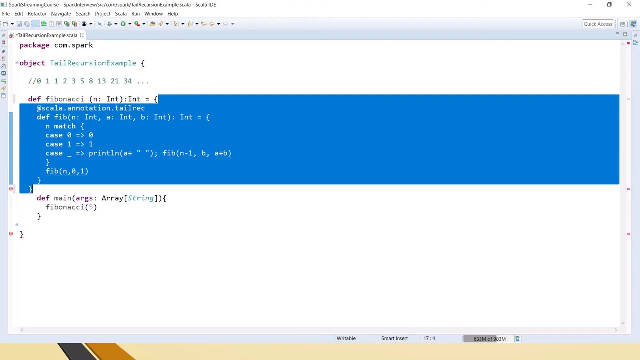 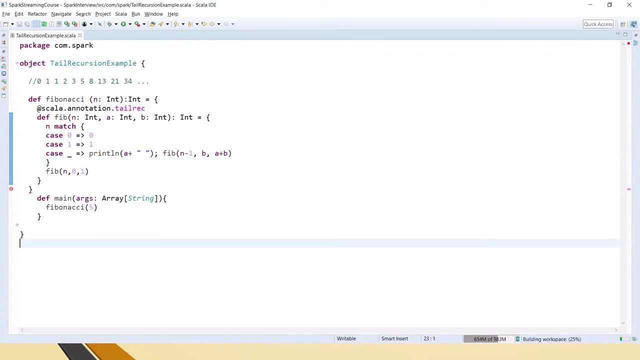 we have started. this is done here, this is done here, this is done here, and inside that we have which is correct. okay, so now here i am passing it. so let's start with the main method. in the main method usually you know that main is seven first will be called. so inside the main method we are sending is at: 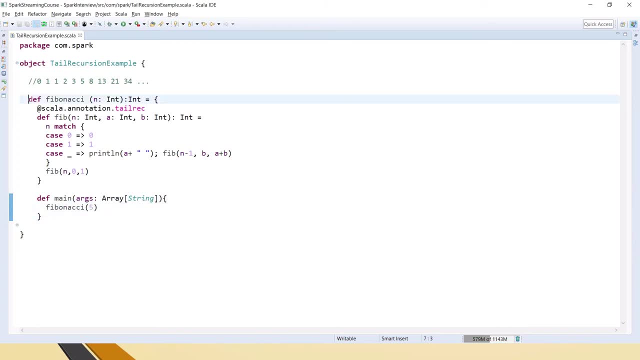 five, and why i have taken a high level function here is for calling any function. anyone would want to send only the number for how many um, um, um numbers in a series they wanted to have. so here we need the zero and one here, but we don't. i don't. 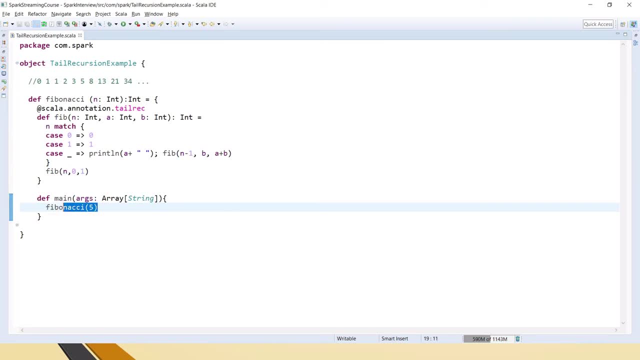 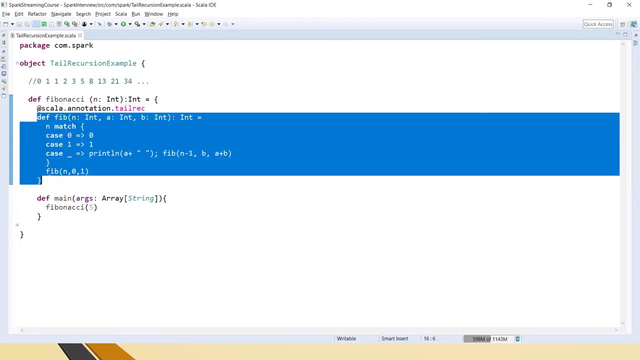 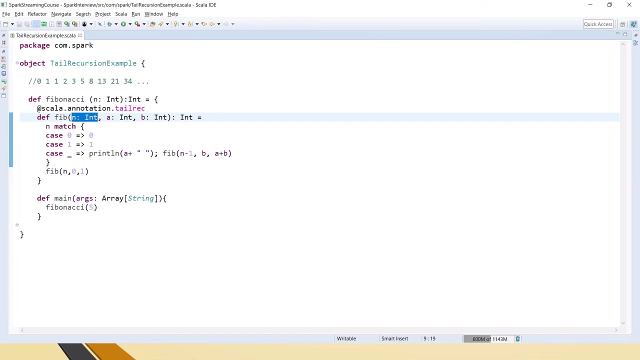 want to send that, uh, show that to the end user. so that's why i have created a function like this. and then here we have the annotation and inside that is the main function for fetching the fibonacci series. so which says that here let's say we, we are saying, here we have the five. no, so once first. 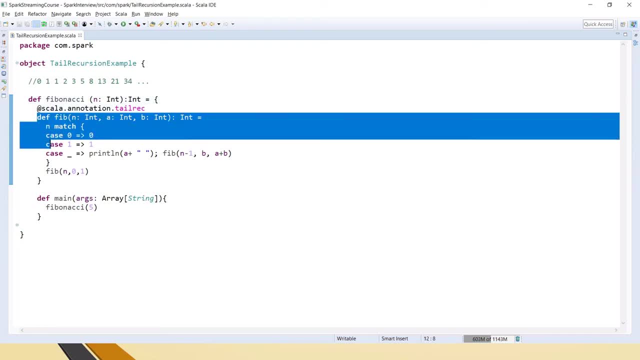 time when it ends, enters to here, it will not execute this correct because it this is just a definition and we are not calling anywhere, and this will become the initial one, which is like five and zero and one got it. so once it will become five, zero one. 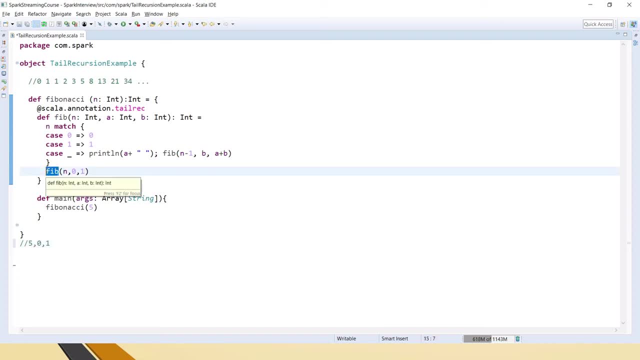 and again we are having a call to this same function. now for the second iteration. it will call here, okay, and now it will call it. it will send five: 0, 1, okay, so now 0. we are matching here with a pattern matching code, so it's not 0, it's not 1, its five, so it will. 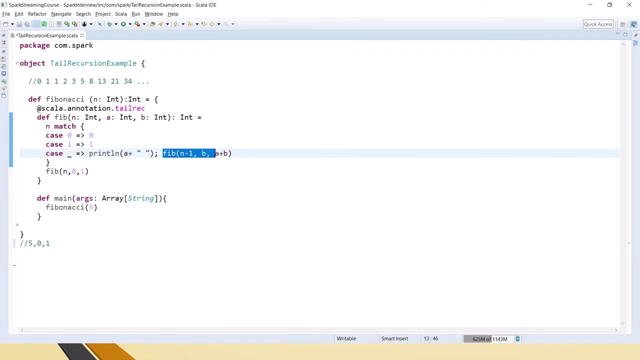 come here, it will search for. it will print a. a is what here? 0. so first it will print 0, and then in the fibonacci series again it is calling the same function again. so fibonacci series, not food, indeed, anyway, again it's a function called to itself. so n minus 1 is what 4, and for here it should be a right. so 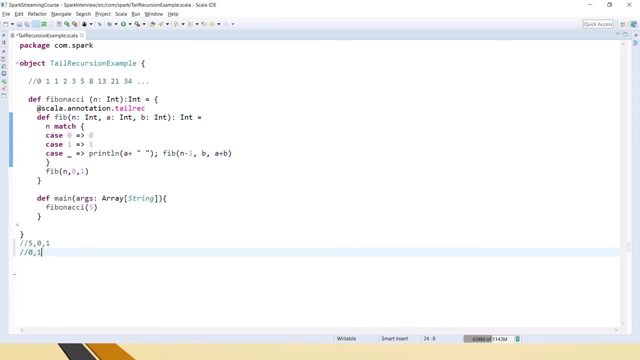 for a we are sending. b means what? 1, okay, and this will become 4. this will become 1 and a plus b, equal to again 1, so which will be sent it as b here and similarly it will come here. now case is 4 in the sense n is 4 here because it we have given it as minus 1, so 4, then again it's 0, 1 will. 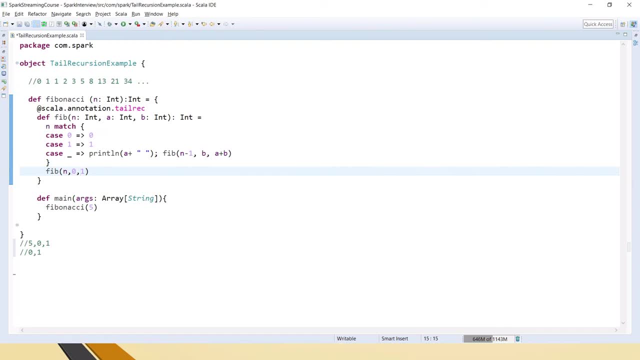 be sent back. so once it is sending, then again it is a is changed to b. now, if you notice here, a means in the previous iteration it has changed to b, so it will become as 1. now it will become a plus b. a plus b means again: 0 plus 1 is 1, now 1 plus 1 equal to 2. so now for b we are sending it. 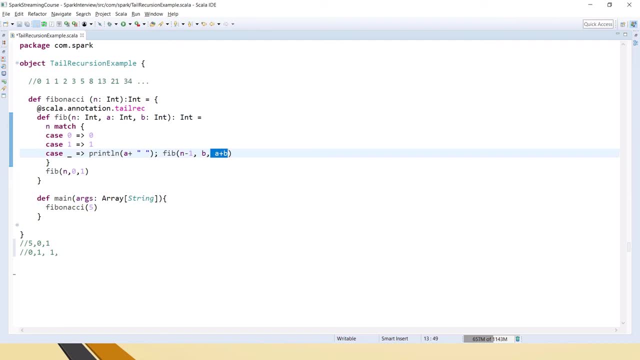 as a 1 plus 1, 2. hope you understood. please make sure that you concentrate this very clearly. it's a bit confusing. if you notice here from the input, we are always subtracting 1 and we are passing b value to the a, and what is b value is which will be computed in the previous 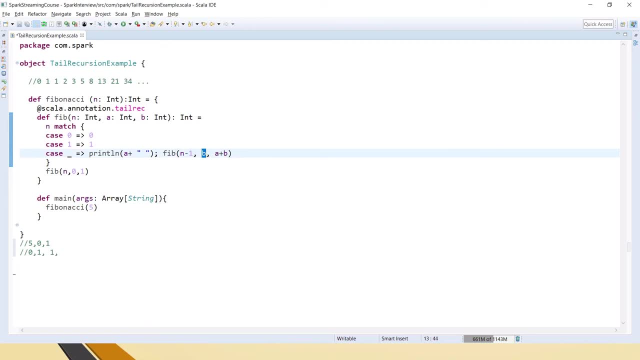 step by summing up a and b. this is where we have the sum, summing up, summed up the total, and this is where we are passing the previous one, like if this is a, then this is b, kind of right. so here b means whatever is summed up in the previous circle and the previous cycle and that